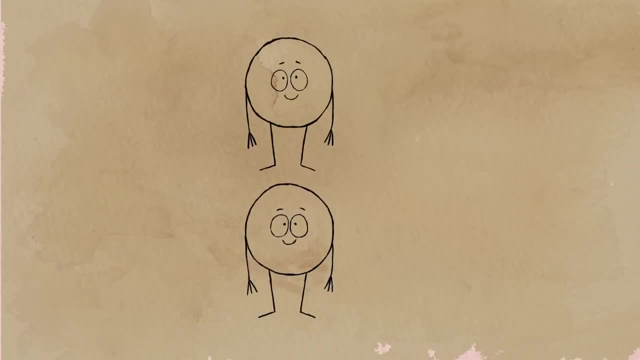 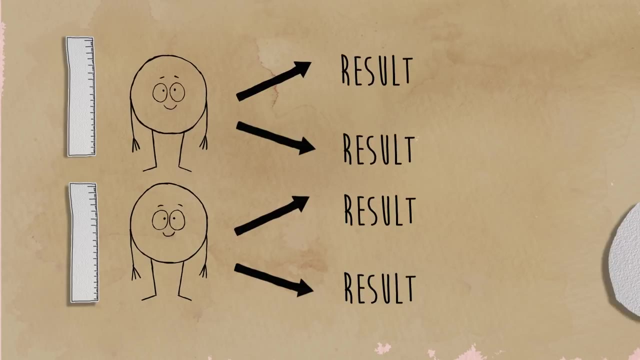 The paper begins by considering a source that spits out pairs of particles, each with two measurable properties. Each of these measurements has two possible results of equal probability. let's say 0 or 1 for the first property and A or B for the second. 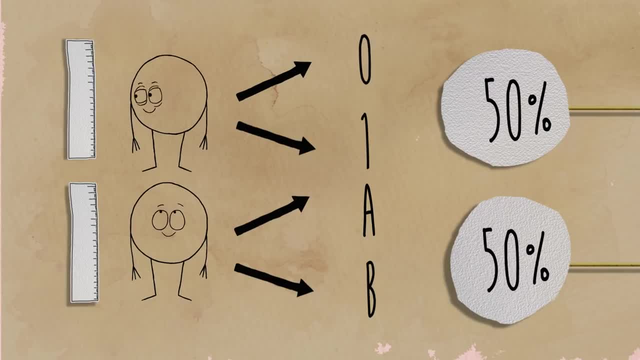 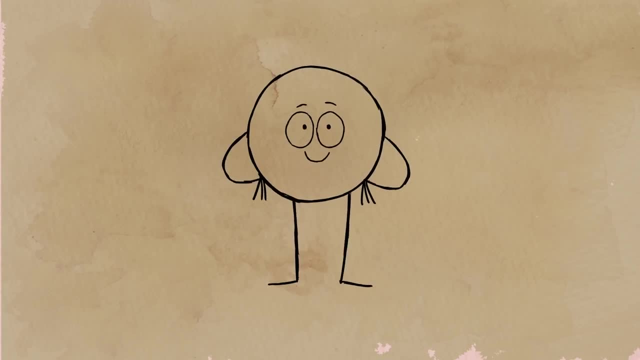 Once a measurement is performed, subsequent measurements of the same property in the same particle will yield the same result. The strange implication of this scenario is not only that the state of a single particle is indeterminate until it's measured, but that the measurement then determines the state. 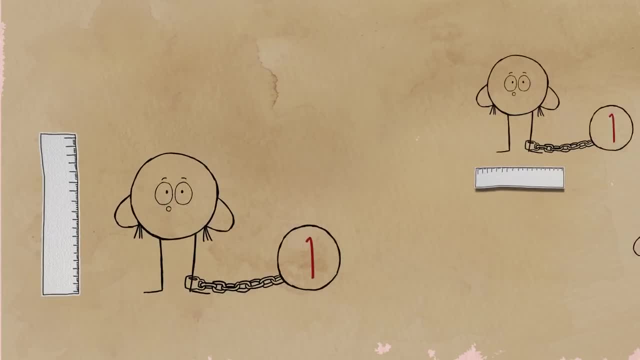 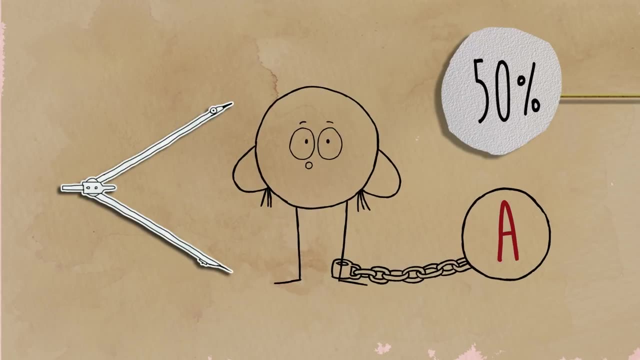 What's more, the measurements affect each other. If you measure a particle as being in state 1 and follow it up with the second type, you'll have a 50% chance of getting either A or B. But if you then repeat the first measurement, 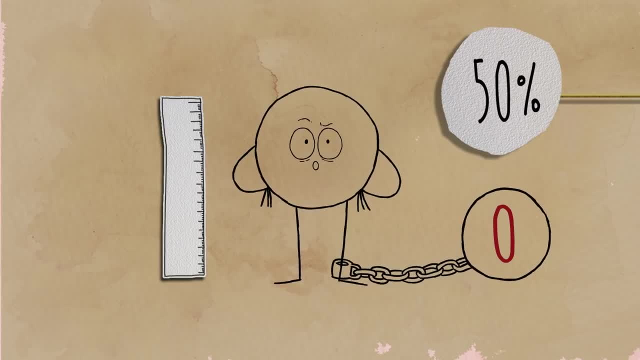 you'll have a 50% chance of getting 0, even though the particle had already been measured at 1.. So switching the property being measured scrambles the original result, allowing for a new random value. Things get even stranger when you look at both particles. 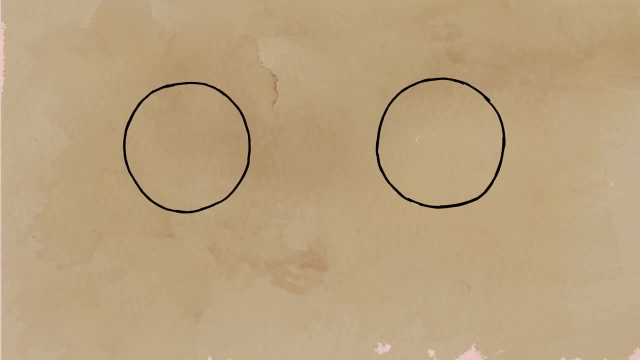 Each of the particles will produce random results, but if you compare the two, you will find that they are always perfectly correlated. For example, if both particles are measured at 0, the relationship will always hold. The states of the two are entangled. 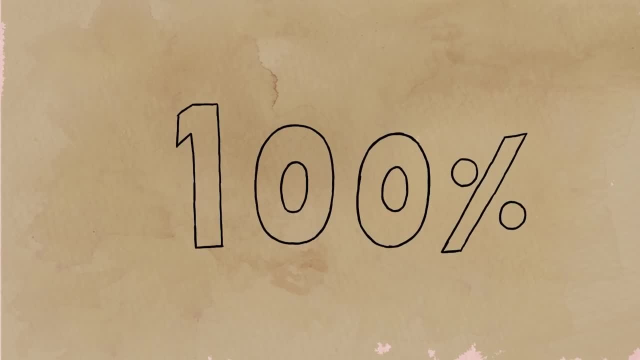 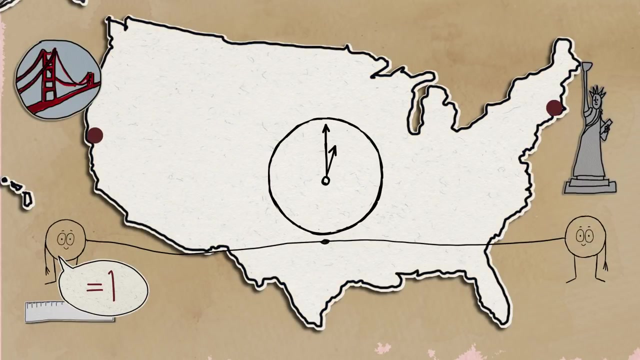 Measuring, one will tell you the other with absolute certainty. But this entanglement seems to defy Einstein's famous theory of relativity, because there is nothing to limit the distance between particles If you measure one in New York at noon and the other in San Francisco a nanosecond later. they still give exactly the same result. But if the measurement does not match and it does determine the value, then this would require one particle sending some sort of signal to the other at 13 million times the speed of light, which, according to relativity, is impossible. 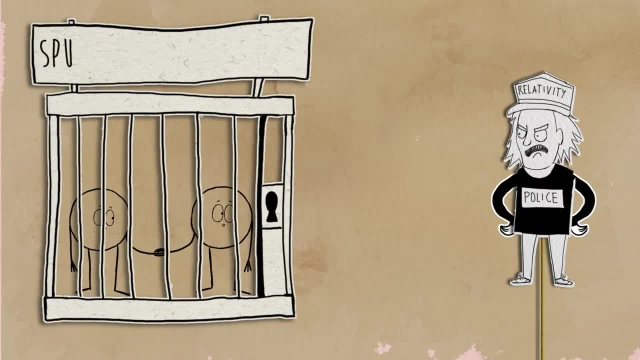 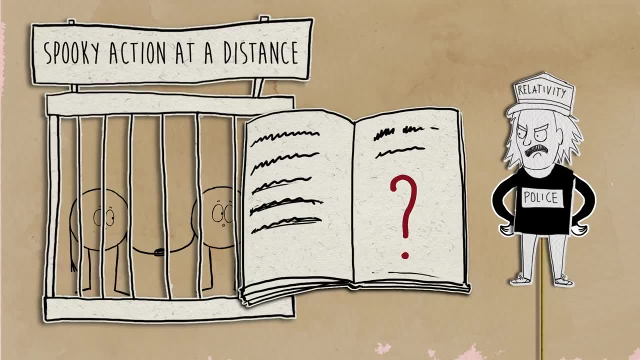 For this reason, Einstein dismissed entanglement as spookhafte Fernwirkung or spooky action at a distance. He decided that quantum mechanics must be incomplete, a mere approximation of a deeper reality in which both particles have predetermined states. 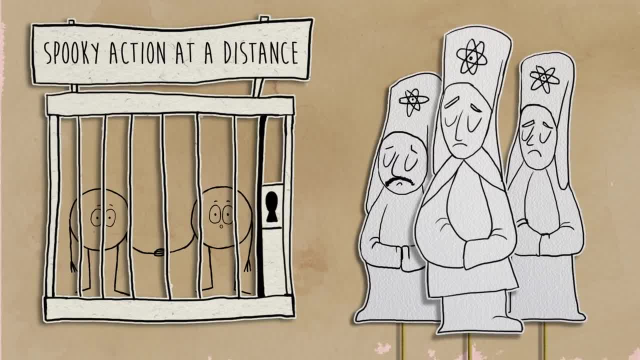 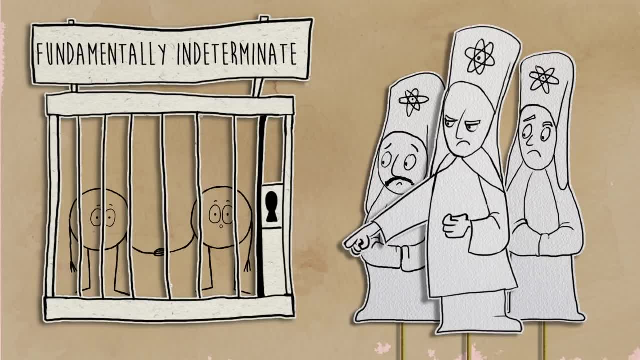 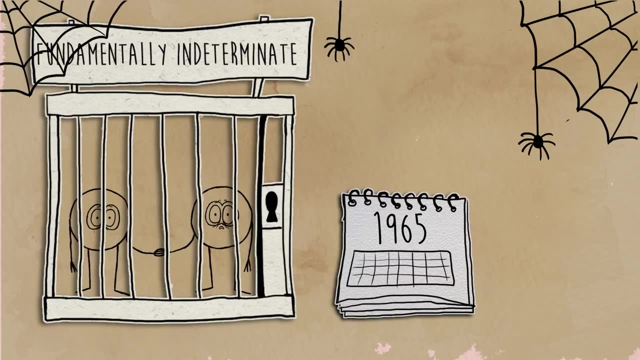 that are hidden from us. Supporters of orthodox quantum theory, led by Niels Bohr, maintained that quantum states really are fundamentally indeterminate and entanglement allows the state of one particle to depend on that of its distant partner. For 30 years, physics remained at an impasse.